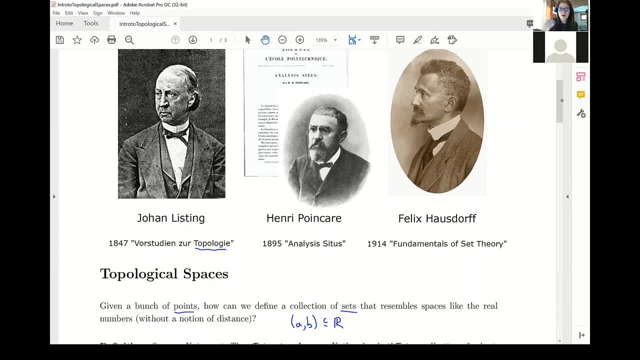 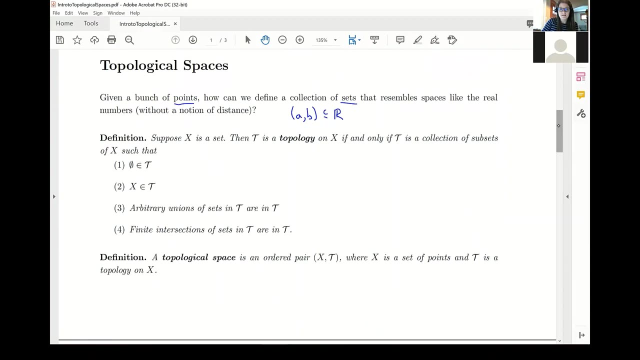 the reals. How can we define a more general space that has a lot of the behaviors of these open sets contained inside of the reals? So this leads us to the notion of a topological space. So imagine we're given a set, and these are our points, and we're given a collection, tau. 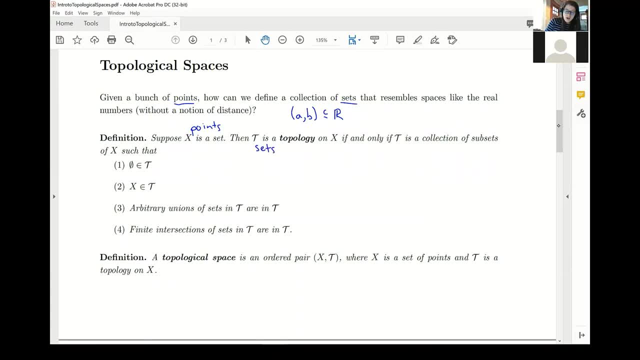 which are our sets. So tau is a topology if it satisfies these four properties that follow. Now we want to think of these in terms of the open sets and the reals. So, for example, if we have a reels, So often we call these the open sets, but we'll see some examples later on that they may not. 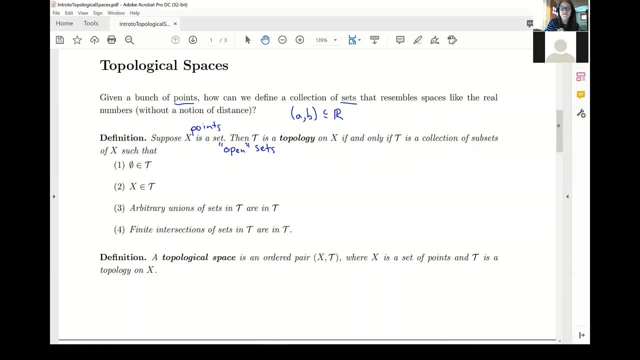 look and feel like the open sets we're used to in the reels. Now, the four properties are that in this collection we must include the empty set, we must include the whole set and if we have a bunch of open sets, we can take arbitrary unions of these open sets so they can possibly 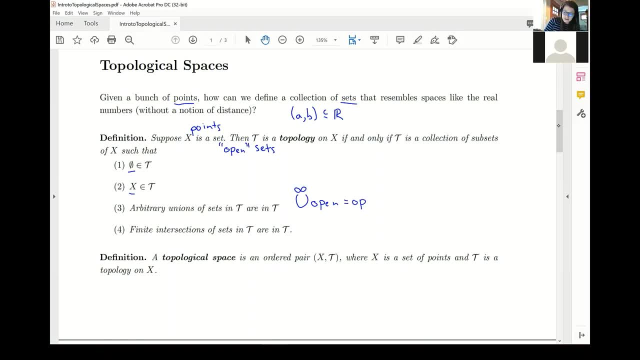 be infinite and we should still have an open set. So a collection of these open sets in tau must also still be in tau. Finite intersections must also be in tau. If you recall properties of the open sets in the reels, they actually do satisfy the 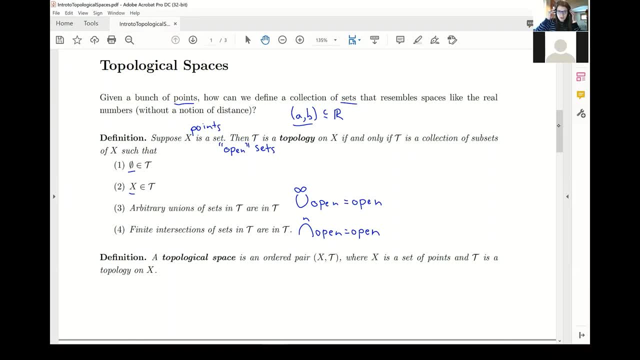 four properties. So a topological space, then, is simply our points together with these sets, and this is where we get the area of mathematics known as point set topology. So if we have this ordered pair, then this defines a topological space. Now I'm going to give an 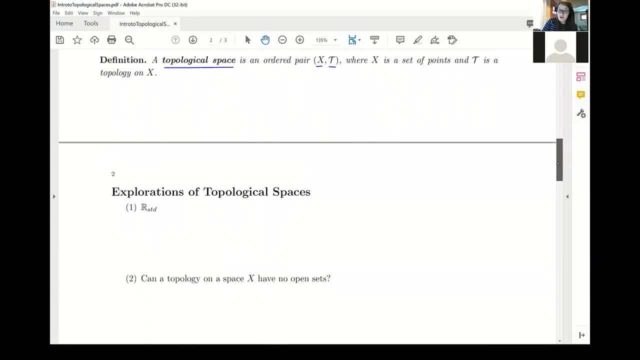 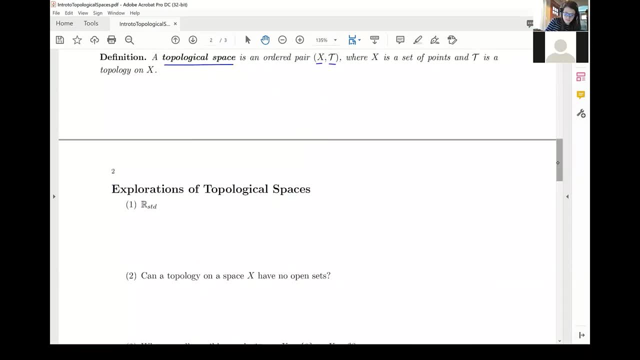 So if we have this ordered pair, then this defines a topological space. So if we have this ordered pair, then this defines a topological space. Okay, so if we think of the reals, we can think of the standard topology on the reals. okay, 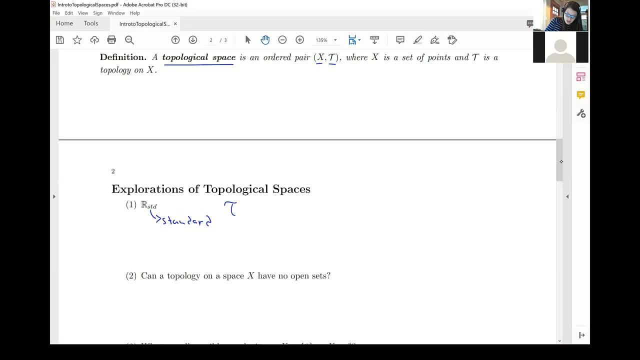 And what we can do is we can form the topology as the collection of these open sets, such that A and B are in the reals and all unions and finite intersections, okay, So if the goal of topology was to define more general spaces in terms of the real numbers, 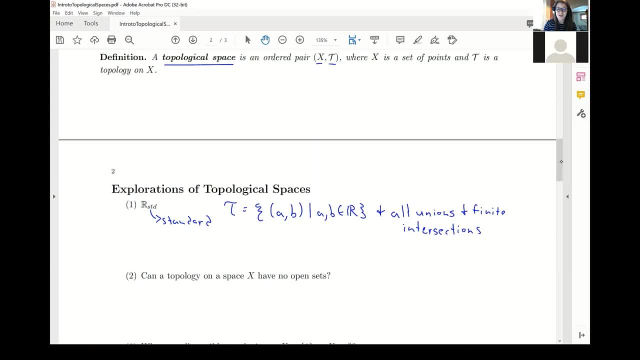 then this better be a topological space itself. okay, So what I've done here is created a collection of elements here in terms of the open sets, and this would actually be what we would call a basis of the topology, where we can take these elements and then throw on. 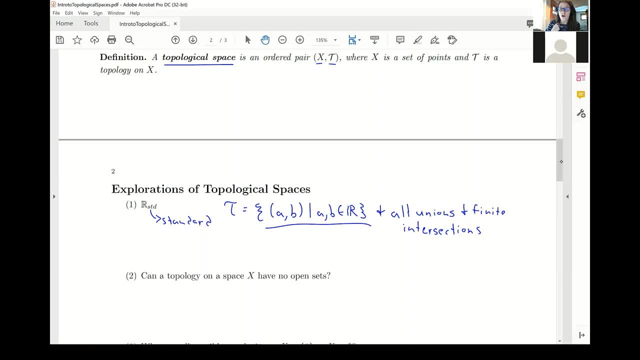 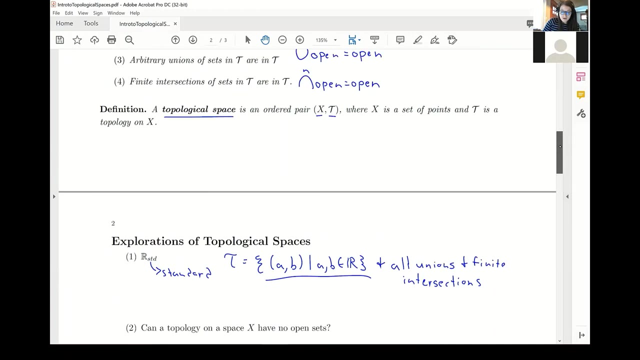 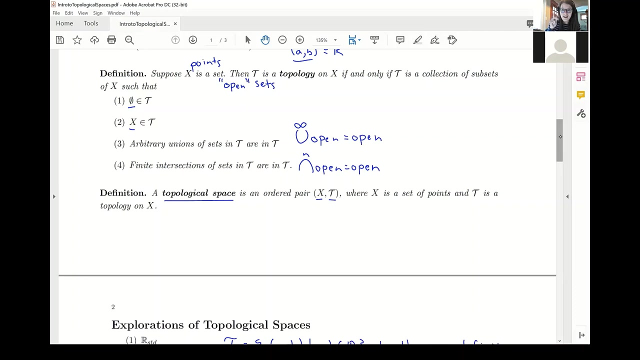 and all possible unions and finite intersections, and it's going to generate all of the different open sets that we could potentially have in our space. Now another question you might ask is: can a topology on a space have no open sets? Well, of course not, because one of the central things in topology is that it must have the empty set. 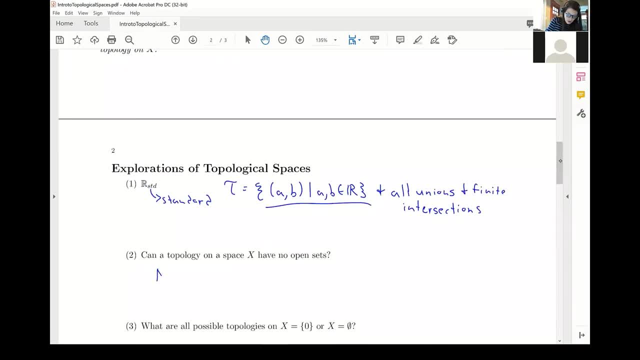 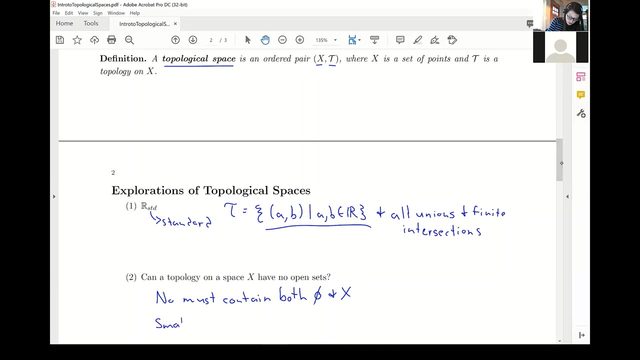 and it must have the whole set. So no, it must. It must contain both the empty set and the whole set. So this sort of leads us to what is the notion of a smallest topology. you can have. The smallest topology on any set is just going to be empty set and the whole set okay. 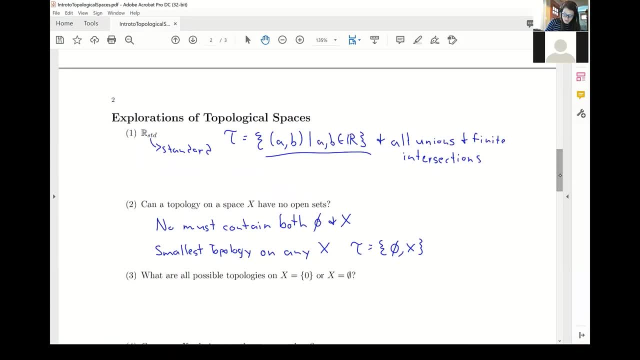 Now imagine I gave you the space of a singleton element. okay, So here we have a singleton element. What is the topology that you can put on this? It turns out that there's only one, and the only one topology is the sort of smallest space. 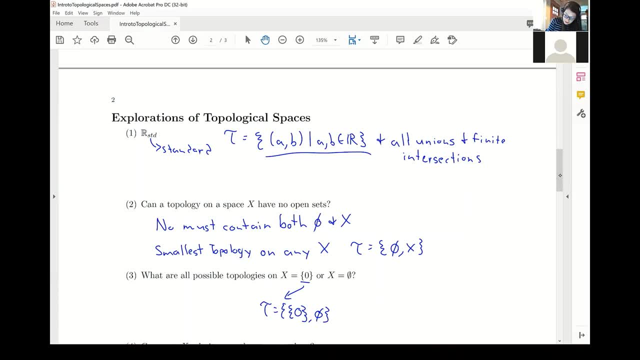 the whole space and the empty set. Similarly, if I gave you that our set of points is just the empty set, then there's only one topology we could put on this, and that is the empty set. Okay, So both of these are sort of these smallest topologies. 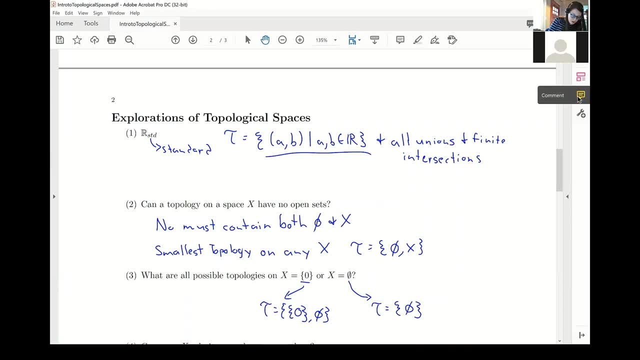 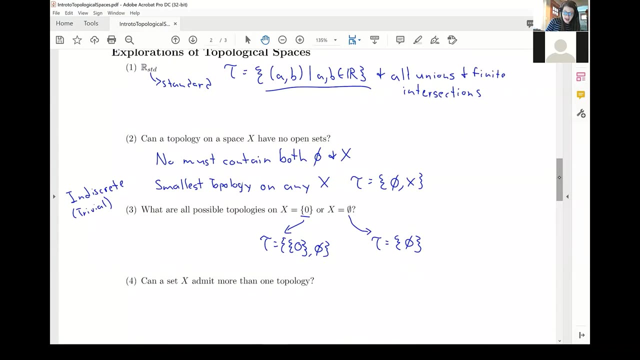 and this is something that we call the indiscrete topology. So this is the indiscrete or the trivial topology. okay, Now another question you might ask is: can a set X admit more than one topology? And hopefully you see, yes, of course. 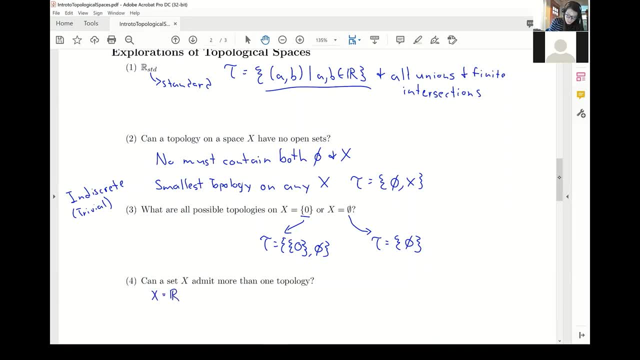 So if our set X is more than one topology, then the set X is more than one topology. So if our set X is more than one topology, then the set X is more than one topology. In the case of this set, if our set X was the real numbers we see, here's one topology. 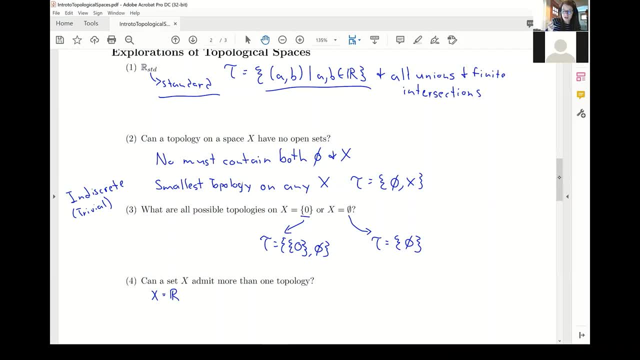 the standard topology determined in the form of these open sets, or we could have say the indiscrete or trivial topology on it. So we could have say: tau equals this, where we have the empty set and all of R. 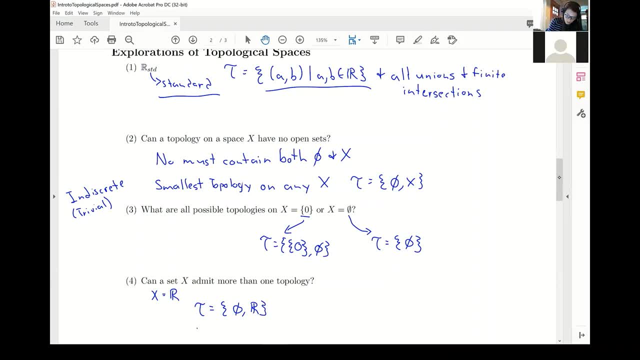 and those are the only things we declare are open. or we could have these a, b, the open intervals in here, and unions and intersections. Okay, So Booth tells us that even though we have the same underlying points, we could have different topologies, creating different topological spaces. 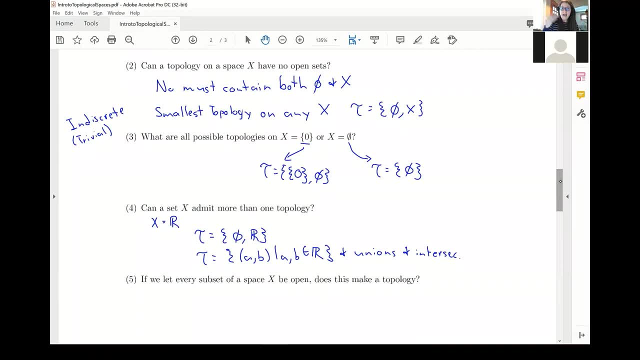 So the question we could ask is: what if we let every subset of a space X be open? Does this make a topology? And if you think of this, every subset of the space X, this would be the power set, and sometimes we use this notation Now. would this satisfy the properties of a topology? 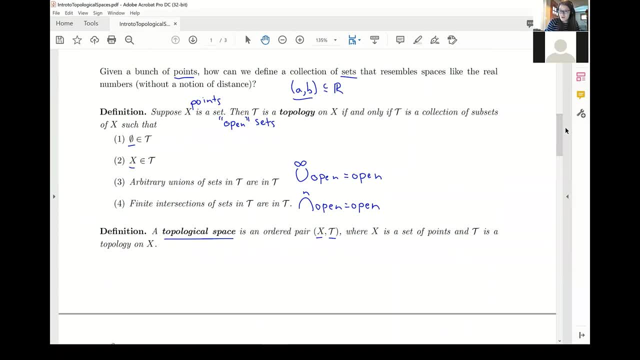 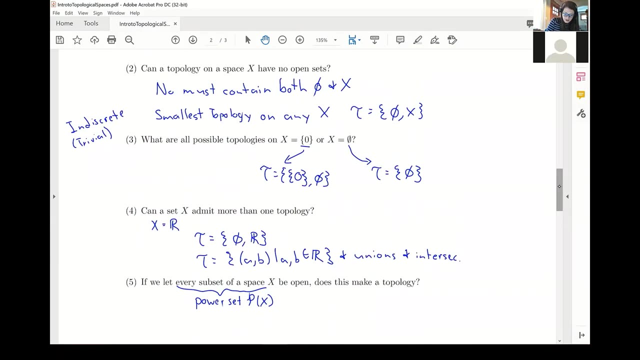 Well, certainly, the empty set and the whole set are in the power set. Any arbitrary unions are going to be in the power set and any finite intersections are going to be in the power set. So, yes, this does make sense. It does in fact create a topology on any set X. 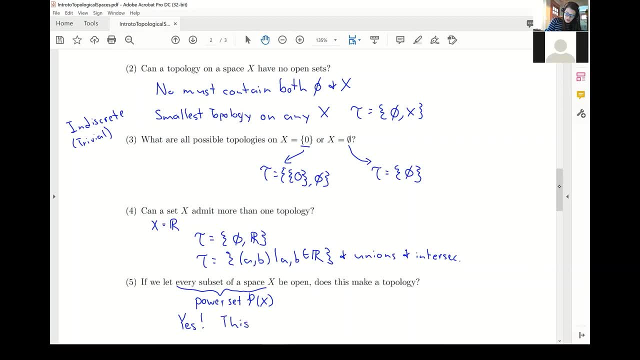 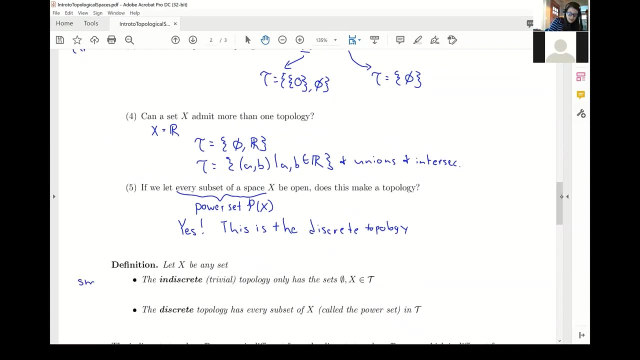 This is what we would call the discrete topology, And I have these formal definitions down here. We sort of have the indiscrete topology, which I like to think of as the smallest topology you could have on any set, and the discrete topology, which 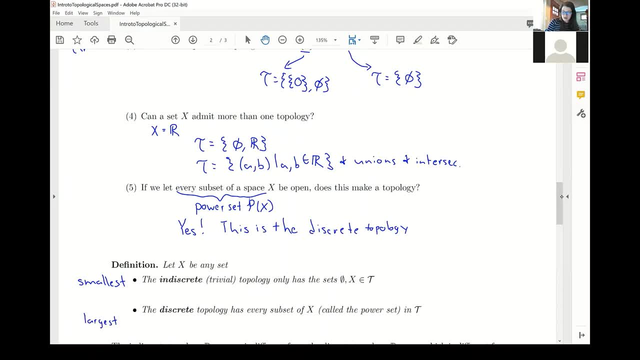 we can think of as the smallest topology you could have on any set. So we can think of as the largest topology on any collection of points. OK, Now, what this tells us is that the indiscrete topology we can think of as being different. 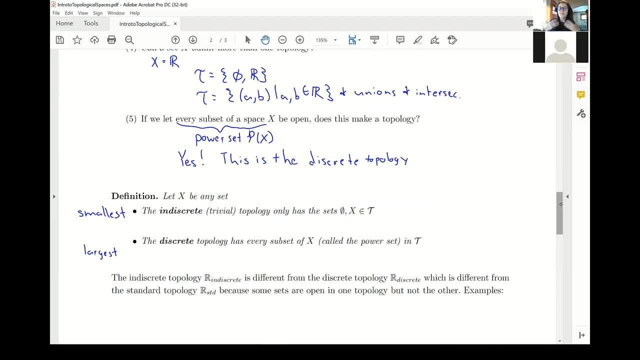 from the discrete topology, which is also different from the standard topology. All of these have different notions of open in their space. For instance, the discrete topology has things like the open set 5, or it could include the interval 0,, 1, or it could include 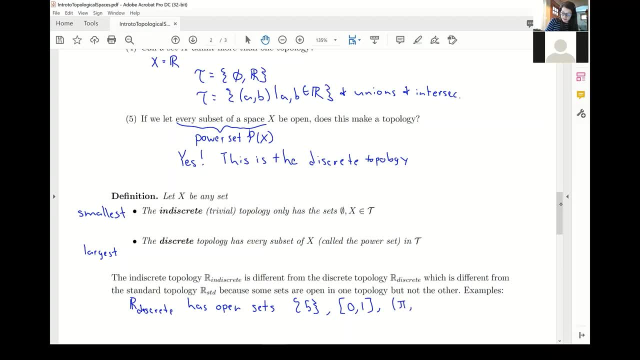 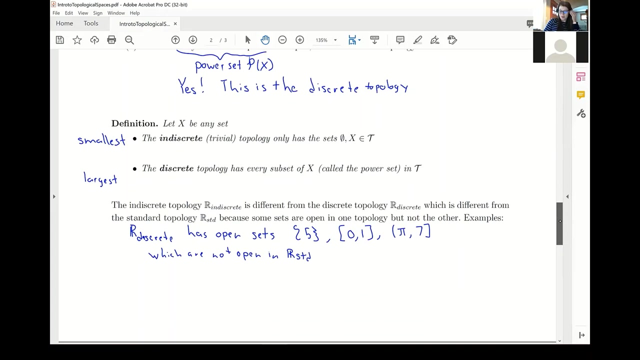 things like pi to 7 with half open intervals. here All of those in the discrete topology are considered open. but these are not open, are not open in, say, our standard. And then our standard has open intervals, our traditional open intervals. Our standard has open sets like 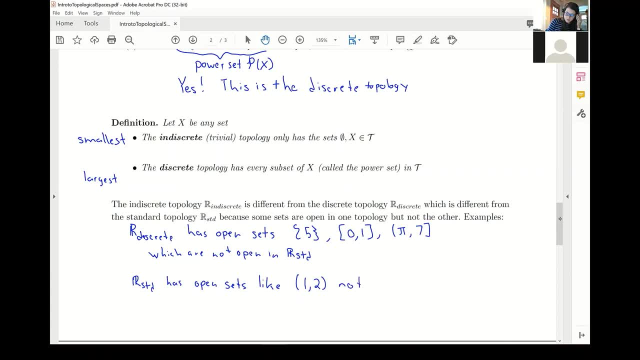 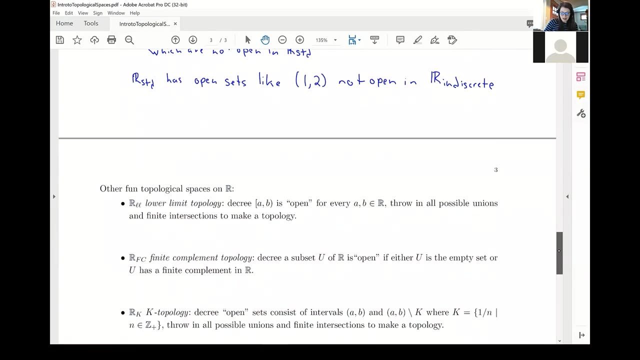 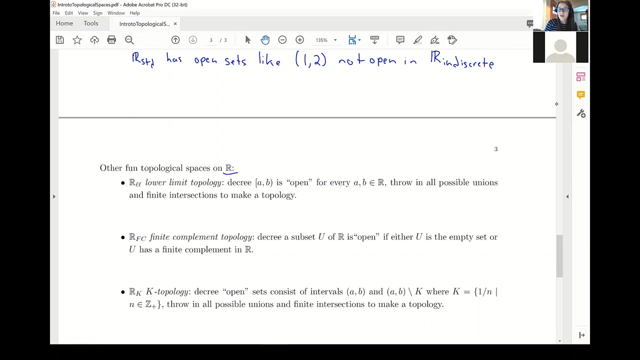 say 1 to 2, which are not open in the industry. Topology tells us that there's lots of different topologies that we could have on any given set of points. Here are some other open sets or different notions of topological spaces we could define just on the single set of points of the reals. 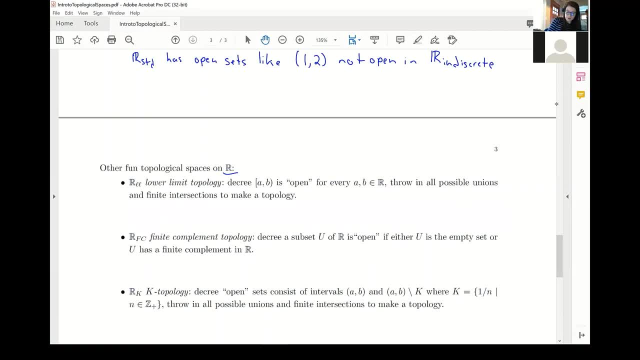 So one is the lower limit topology. It turns out if you take any element like 1 to 2, half open interval, like this, then you say these are going to be defined to be open. We can throw in all possible unions and finite intersections. So elements like this would actually form a basis for our topology. 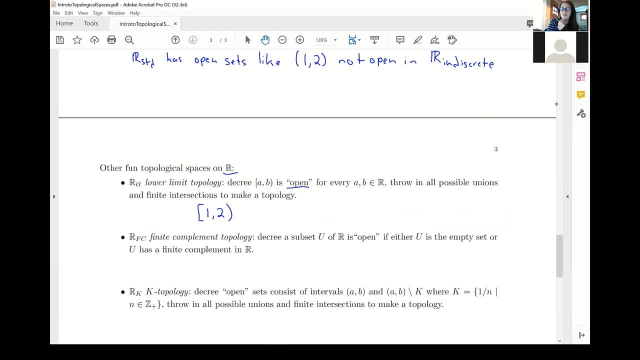 It turns out that this will actually satisfy those four properties that I listed above. Go check it out for yourself. The most interesting topology on the reals is the finite complement topology, where we can take the real line and imagine we exclude the finite number of points. Now 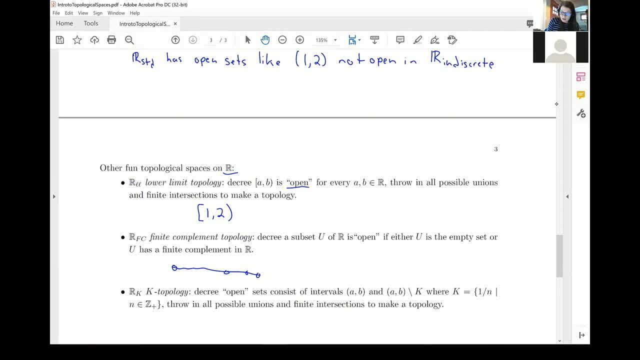 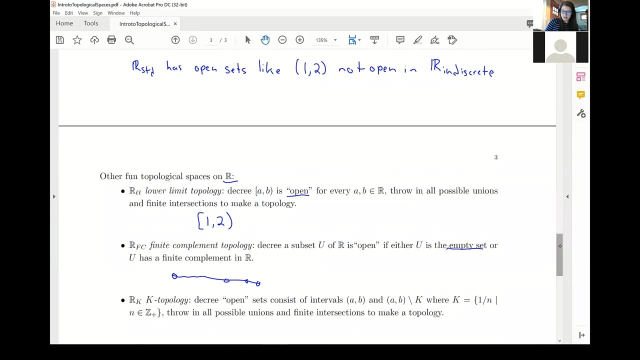 sets like this or the empty set are defined to be our open sets in the finite complement topology. Again, it satisfies those four properties from above. And then the last topology I'll introduce is the K topology, And these we have open sets. 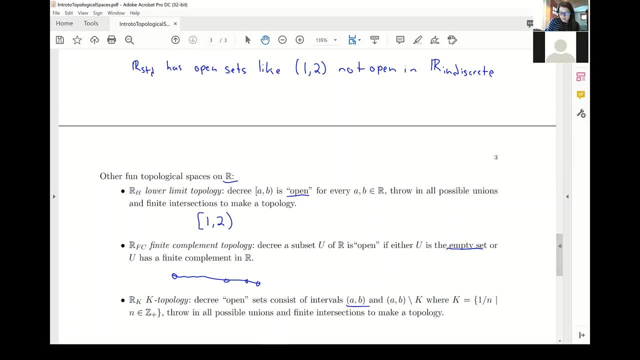 which are just our standard topology. And then the last topology I'll introduce is the K topology: open intervals or open sets, excluding some elements which we'll call k. So think of this as the set minus And the elements k are the one over n, where n is a positive number. So if we had just 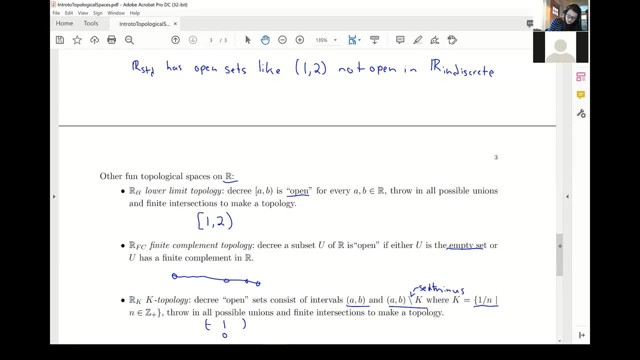 some standard interval and imagine this is zero in our interval. we're going to exclude all of these points along here. Okay, So those are what's defined to be open. So hopefully you see that all of these satisfy the properties of a topological space and in particular a topology. 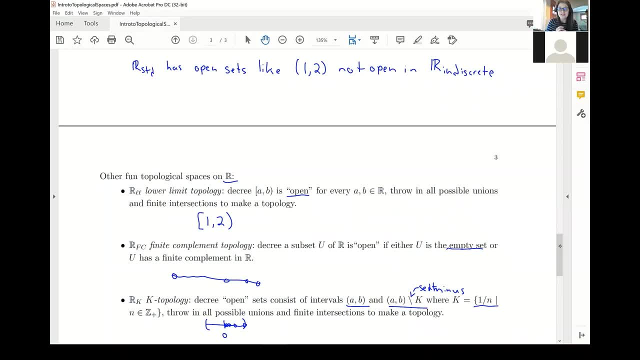 but they look and feel very different. So these open sets may not be our traditional notion of open, but they still satisfy the same property. So the key takeaway is that a topological space is a topological space. So if we have a topological space, we have a topological. 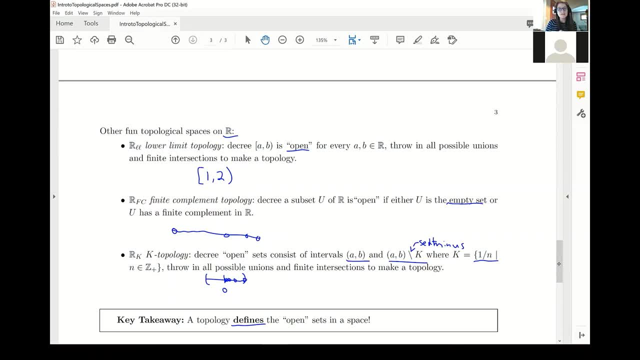 space. So if we have a topological space, we have a topological space. So if we have a topological space, So if we have a topological space, we have a topological space. So a topology actually defines a open set in a space and once we have this definition we can get a topological space.